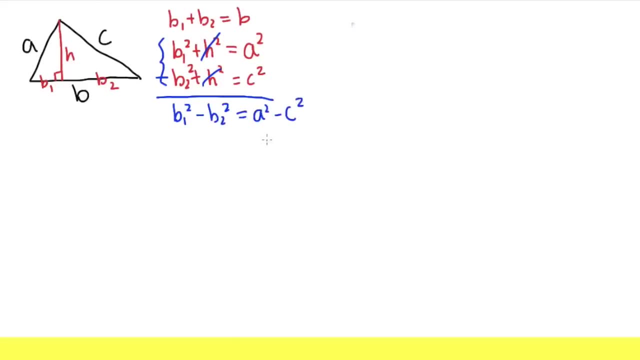 that's equal to A square minus C square. That's pretty good. And notice, this is the difference of two squares. So of course we can factor it B1 minus B2 times B2.. I mean B1 plus B2,. 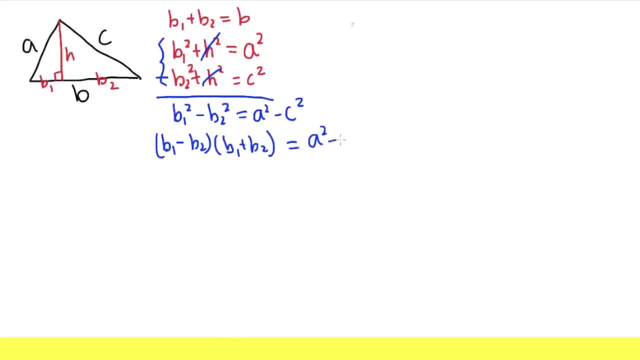 like this, and that's equal to A square minus C square. I am not factoring out the right-hand side, because we notice the left-hand side here. this right here is nicely equal to just the B right, And let's divide the B on both sides. So in another word, we can see that B1 minus B2 is nicely equal to. 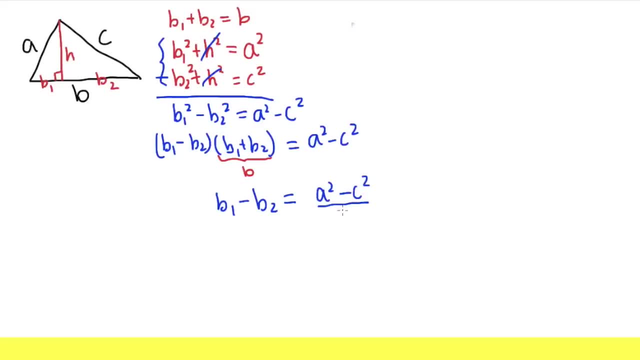 A square minus C square all over B, And you can see that the right-hand side is just in terms of A, B and C, which is pretty good, And we can make it better, because if you look back to this equation, 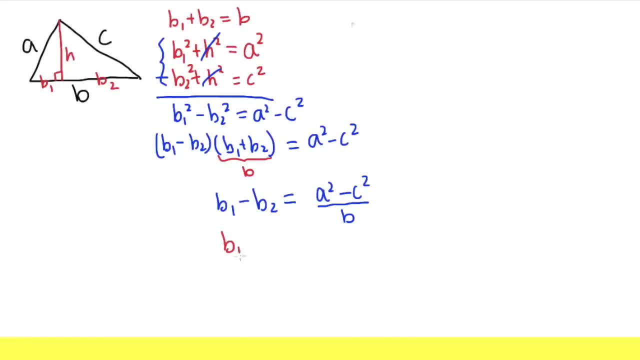 we have B1 plus B2 is equal to B. Let me just put that down And I am just going to add the equations, because this way we can actually get rid of the B2, right, This and that will be cancelled. So let's work with this first. Well, 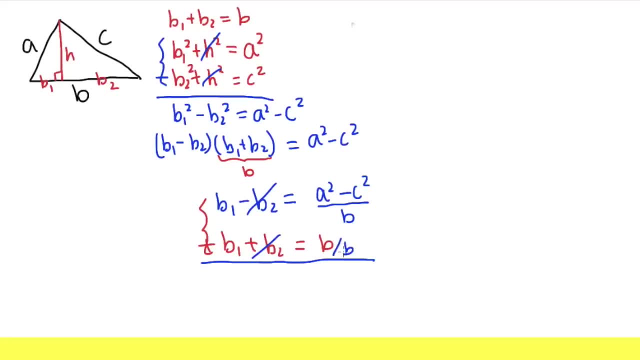 let's get the common denominator. So this right here should be over B, and I need to multiply by this. This is B square plus this and that. Let me write it as A square plus B square and then minus C square over B. Okay now the left-hand side: B1 plus B1, just 2B1.. Let me divide the. 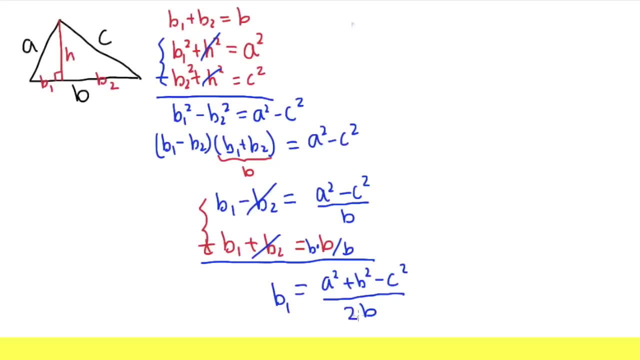 two on both sides. So I get B1. equals this over 2B, like that? yeah, So that's what we have for B1. And perhaps we can write it down right here just for some notes. Hmm, Okay, I have B1.. By. 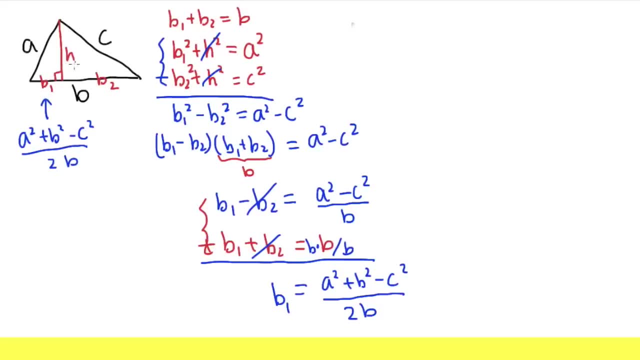 still need to find H. What's the connection between B1, H and A? Well, it was right here, right? So if you look back here, we can subtract the B1 on both sides In another word: H square. 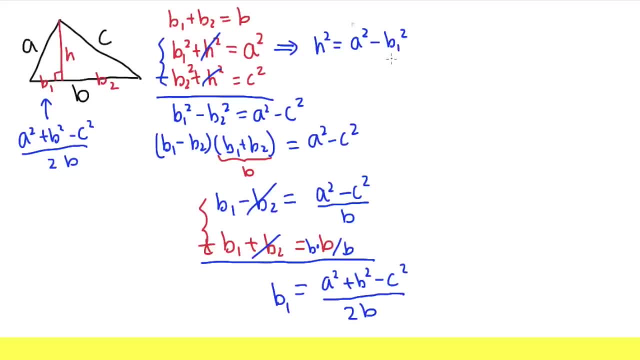 equals A square minus B1 square, And of course we can just take the square roots on both sides. Of course, just do it with the positive square root, because we are doing geometry. So H is equal to this right here. So that's pretty good And I'm going to write that down right here for. 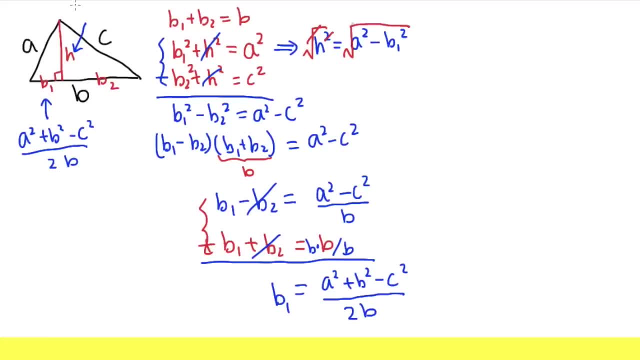 you as well. So H is nicely equal to square root of A square minus B1 square. That's good, And you see, B1 is in terms of A, B and C. I can just put that down right here And that's pretty much. 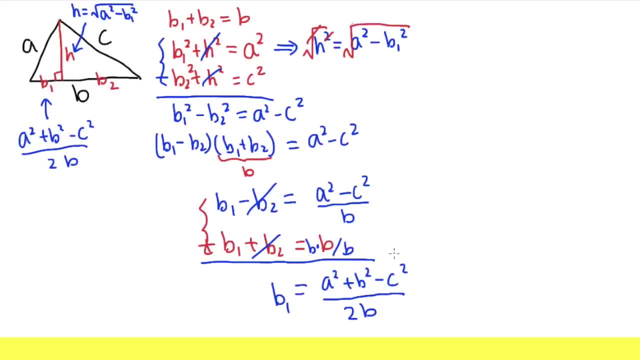 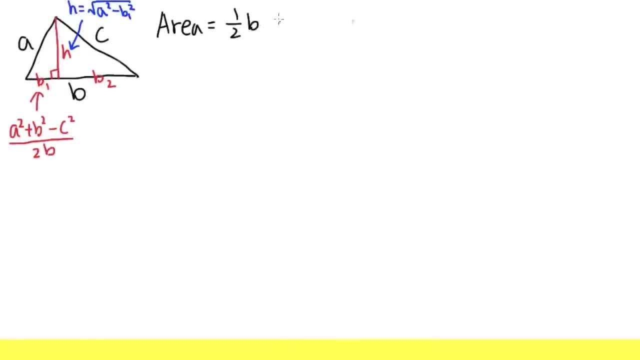 the idea right. So let me clean things up right here and I will do the next part. So now here is the DO. The area of a triangle, of course, is equal to one half times base times height, And of course we have seen that. 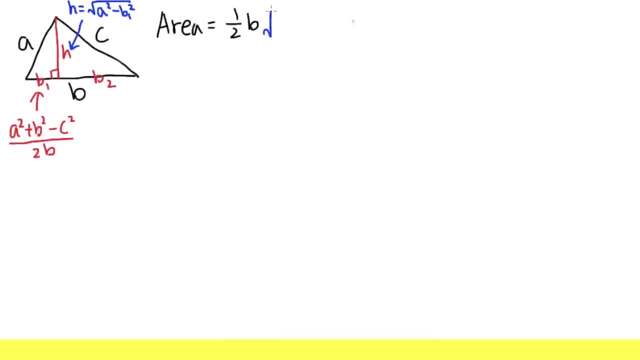 Earlier H is equal to this. So we'll just open a square root And inside here we have A square minus B1 square And we know B1 is equal to this And that's so nice, because B1 is in terms of A. 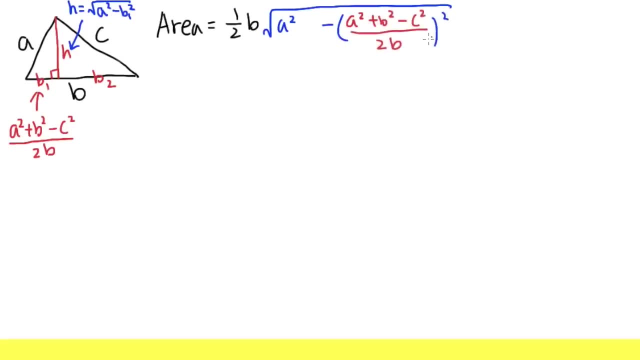 B and C, And now we can just write that down, And now this formula is actually so so, so nice, because the area of a triangle is already, in terms of A, B and C, right. However, this is not how. 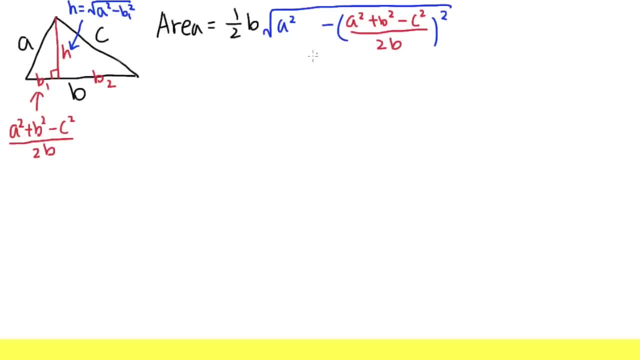 to do some more algebra for you guys in order to get to the form that we want, right? Okay, We can combine fractions inside. Notice, on the bottom here is 2B, and then we have to square, that meaning that we actually have 4B square. So for this I will have to multiply the bottom and the. 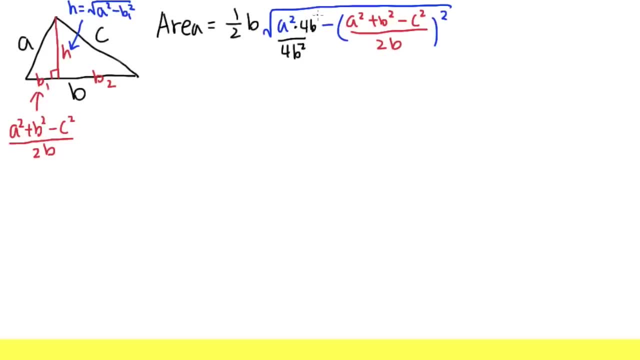 top by 4B square, so they will have the same denominator. So that's pretty good, And let me just continue. Let's have the 1 over 2B all the way in the front and then the square root Both. 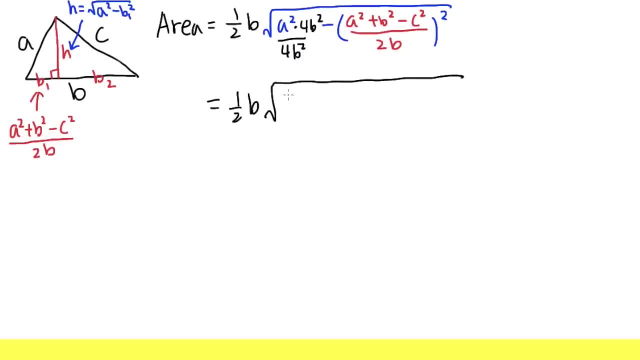 then will have the 1 over 4B square. So I will just write that down first, 1 over 4B square, And then notice that for this part is 4A square, B square and a minus. This is something square. 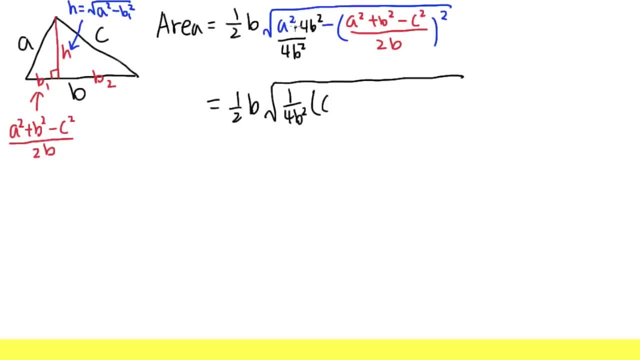 Hmm, I think it's a good idea to write this as parentheses, with 2AB inside and then square and then minus. For this I will keep it A square plus B square minus C square and then square, Because this way we can actually use the difference of two squares to factor out inside. 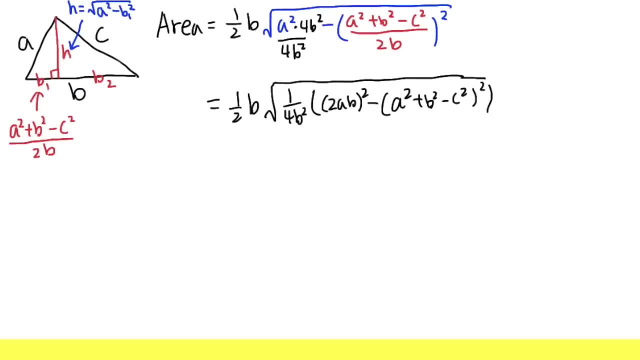 right, Which is very nice. Now you notice that we have the 1 over 2B in the front. huh, Let's invite them inside of the square root house, And when you do that, be careful though. 1 over 2. 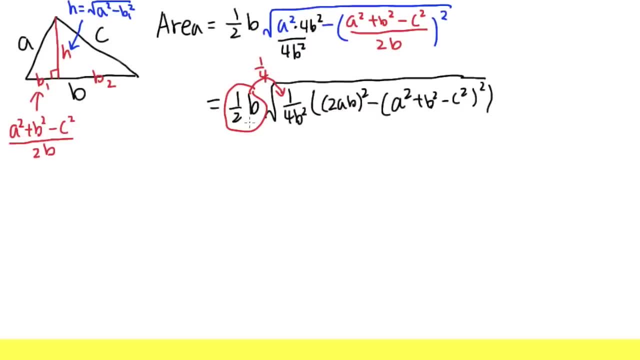 inside of the square root becomes 1 over 4.. And then the B on the outside inside becomes B square right. So you can see everything will be inside And 1 over 4 times 1 over 4, that's 1 over 16.. B square and. 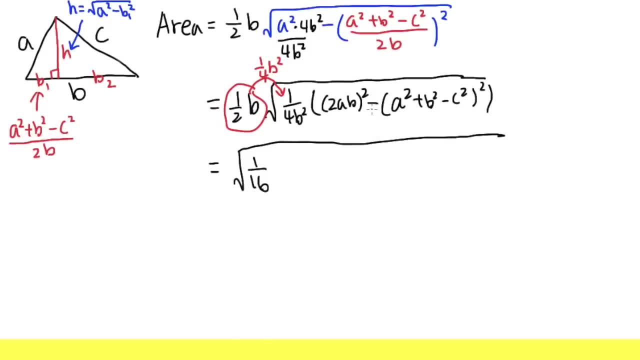 over B square, they cancel out. And now we can focus on this: Factor it out with the difference of two squares. Notice, here is the first term and this is the second term. Now let's go ahead and continue. Parentheses minus another parentheses. That's the first factor, And then another factor. 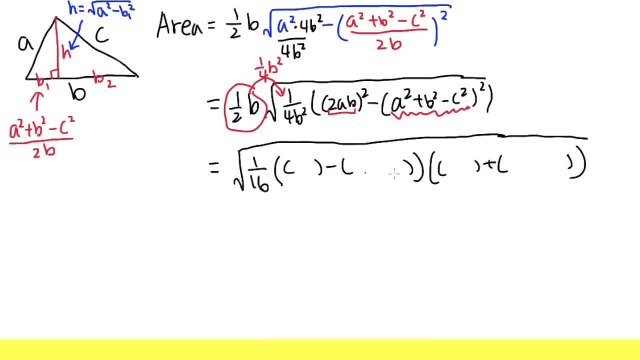 plus parentheses, plus the second parentheses. Well, what's inside of the parentheses? Of course that's just doing everything. Hmm, very nice, huh. Now the question is: can we do more? Of course, Notice. for this part, though, if you distribute the negative from here to here, you will notice. 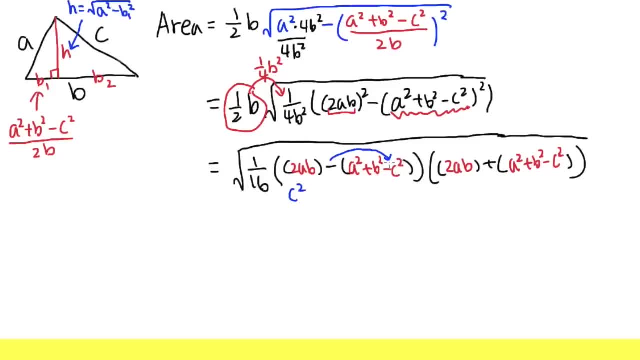 that we actually get C square first, right, And then if you distribute, distribute, you actually end up with minus, and then we get A square and then minus B square, right, And this right here plus 2AB, like. so This is the perfect square, which is very nice. okay, And for this part though, 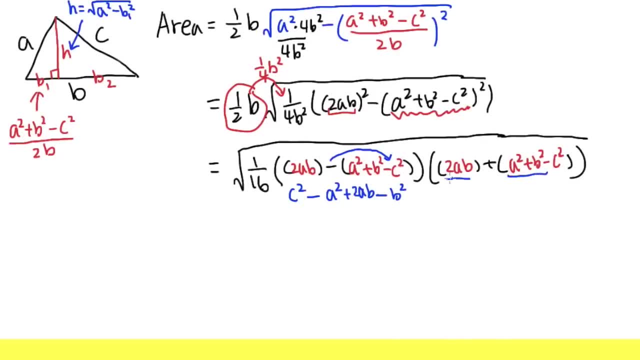 if you focus on 2AB and also this, well, that's also a perfect square. Let me write it down. first, We will keep it as A square plus 2AB and then plus B square, And in the end here we have the. 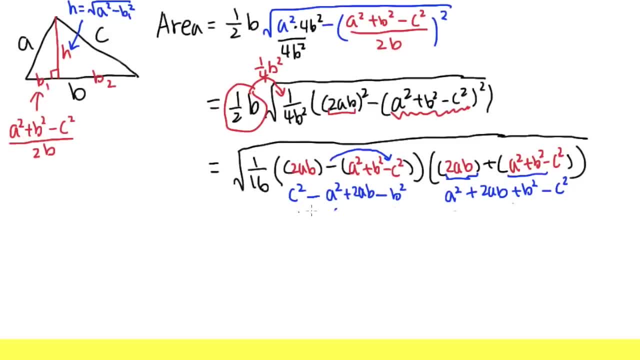 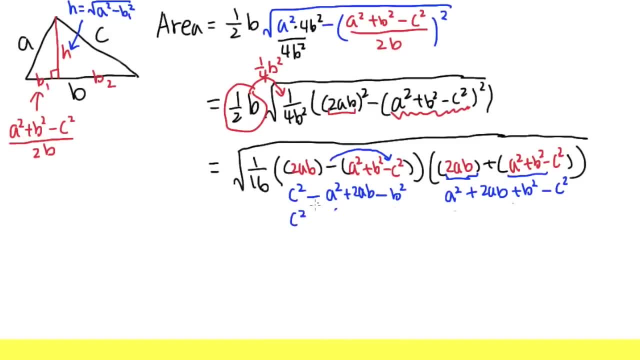 Now we can factor more, because here is C square and I can factor our negative first. If we do that here it becomes A square minus 2AB plus B square. In another word, that's A minus B and a square. 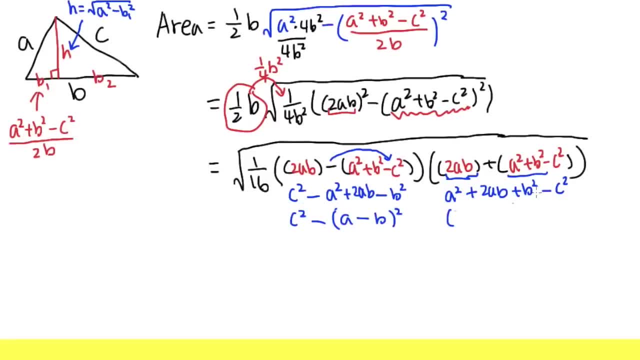 Very nice, huh? And then here we can of course factor the first three terms. It's A plus B square and then minus C square. This is the difference of two squares, and of course this is also the same thing, right? So? 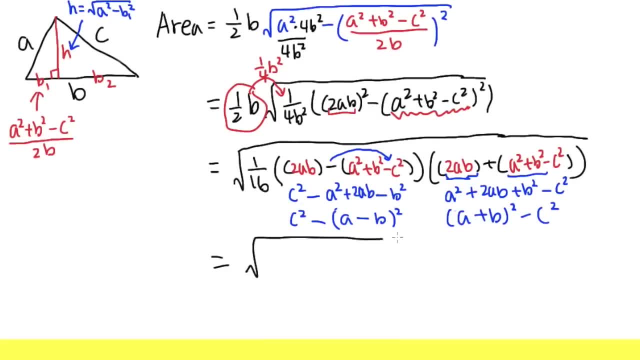 I think now it's a good time for me to write down the square root again. Let me not put down the 1 over 16 yet. Let me just look at this and then factor it for you guys. Right here we will have C minus this and then C plus that, right. 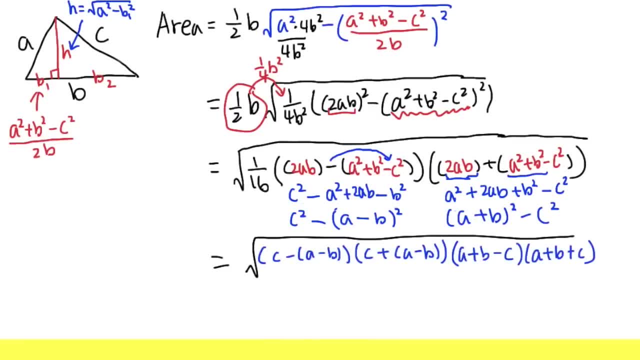 And then for this right here. of course, you can do the same thing. Now. here is the time to take care of the 16. And notice that we happen to have 1,, 2,, 3, 4, 4 factors, and 16 is precisely two to. 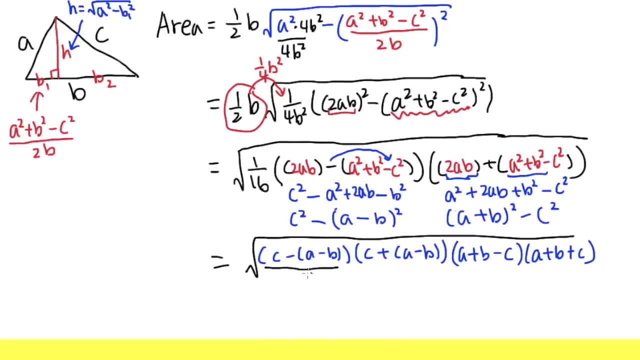 the fourth power right. So I will write down the 16S, This right here, over two, and then over two, and then right here, and then right here. Very nice, Now, here we have A plus B plus C over two. 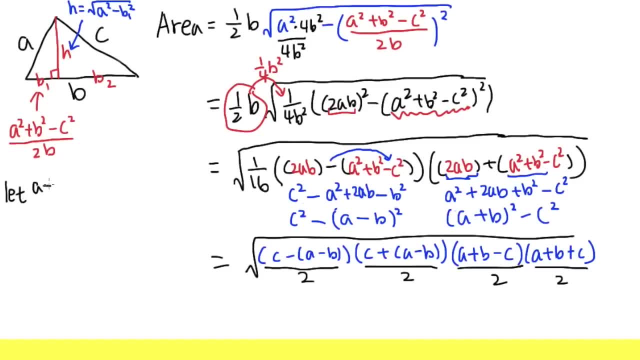 I'm gonna code that to be S, So let me just write that down. Let A plus B plus C over two to be S. And this right here is what we call the semi-parameter, because A plus B plus C is the parameter of that triangle and divided by 2 is, and divided by 2 is, of course, the semicolon. So 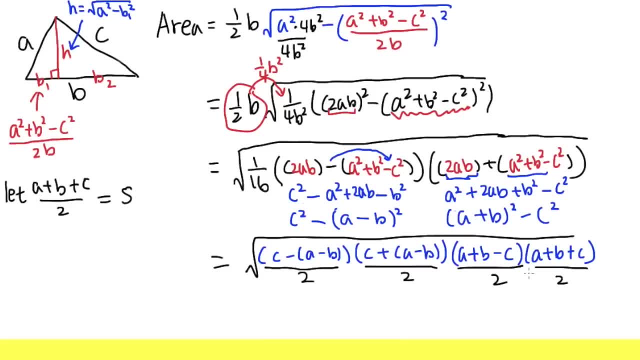 version of it. very nice, right? hmm, this right here is s. how about this, though? well, it's actually really nice as well if we have a plus b, minus c over 2. this right here, have a look. in fact, it's the same as saying a plus b plus c over 2, and we just have to minus c, and you see this right here. 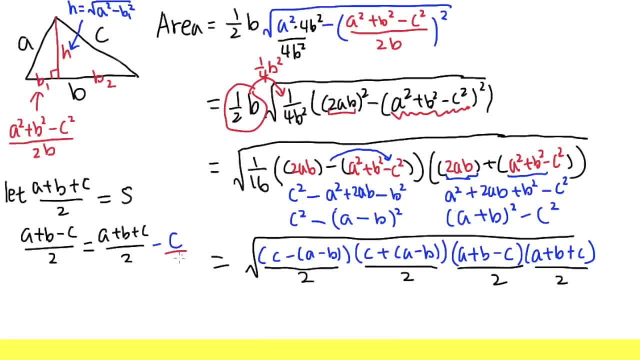 works because, of course, to get a common denominator i need a 2 and a 2. c minus 2 c is precisely the negative c, which is very nice, right, and the rest can be done with the same way. so i'll let you guys verify that yourself. finally, i will tell you this right: here is s: 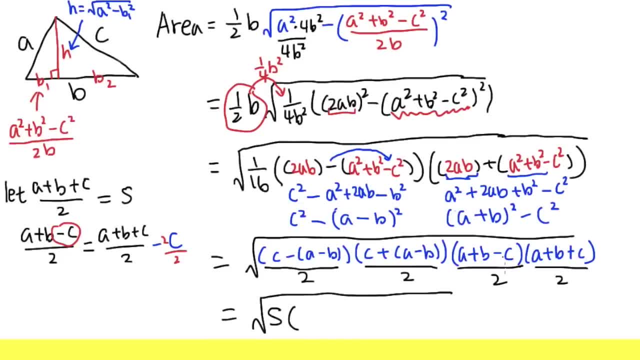 and then next we have the s minus c, and you can imagine we have s minus b. and then next we have the s minus c, and you can imagine we have s minus b, and then next we have- And this right here is S minus A. So all we have to do is just write that down. 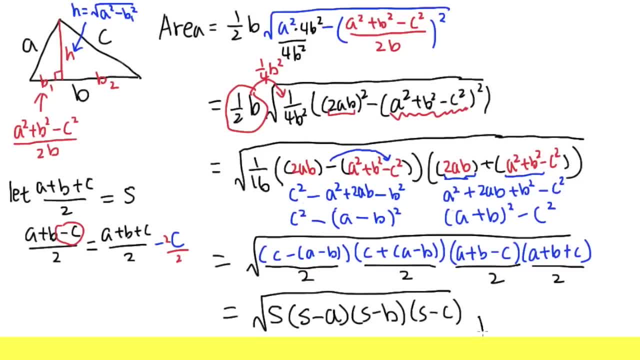 So, ladies and gentlemen, this right here is the Hiron's formula for the area of a triangle, And this is a proof. So I will draw a box and shade this in.